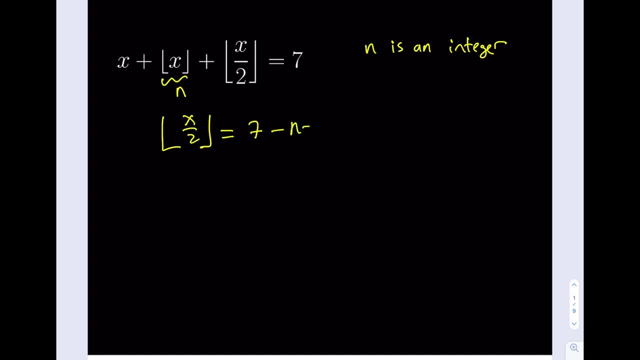 7 minus n minus x: Right, Awesome. Now we have a conclusion here. Since we assume that the floor value of x is equal to n, this means that x is between n and n plus 1. Half closed interval: Right, Because n is an integer and x needs to be in that interval. 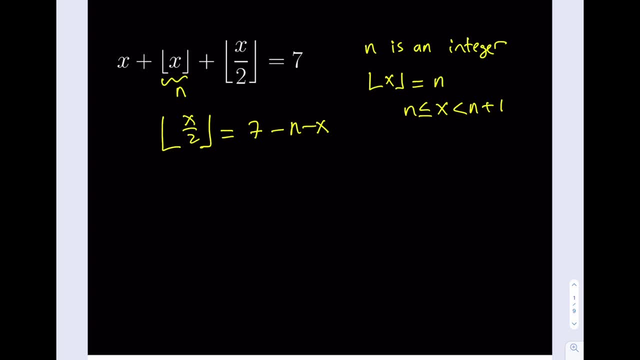 Cool, Now this also has a meaning, obviously, Right. So we can safely say that x over 2 needs to be, according to this equation, needs to be between 7 minus n minus x and 8 minus n minus x, So one more than that, Right, Okay, Cool. Now what does this give us? 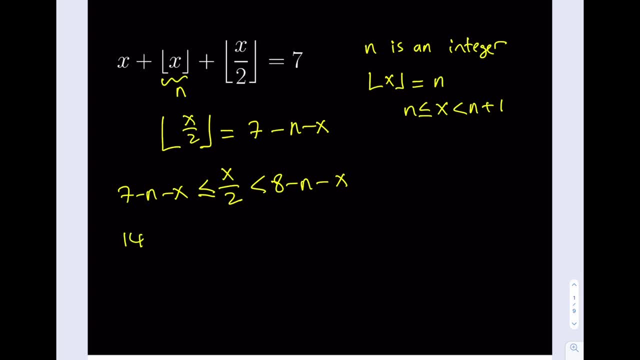 Let's go ahead and multiply everything by 2.. That should give me 14 minus 2, n minus 2.. 2x less than or equal to x, and that's less than 16 minus 2, n minus 2x. Again, I'm multiplying. 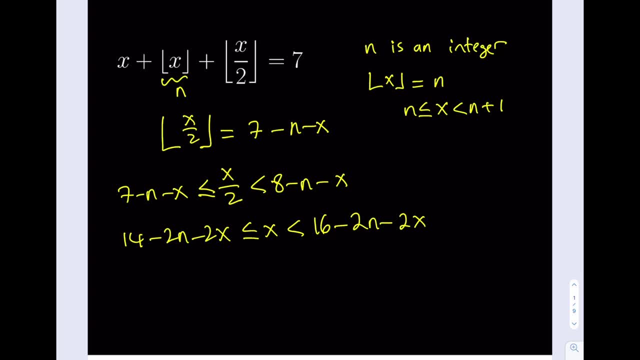 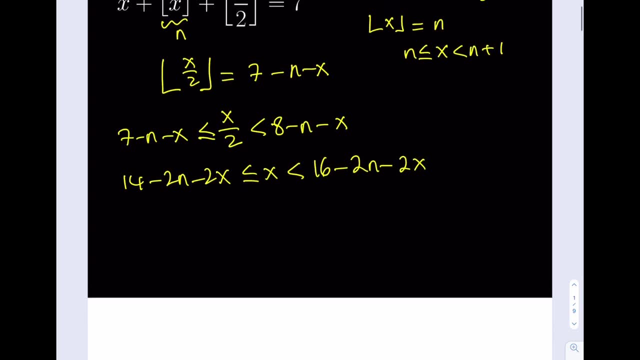 everything by 2.. Right, Okay, Cool. So this, this is fine. I got an inequality for x like an interval, but I have x's on everything, So let's go ahead and put all the x's together. Let's add 2x to. 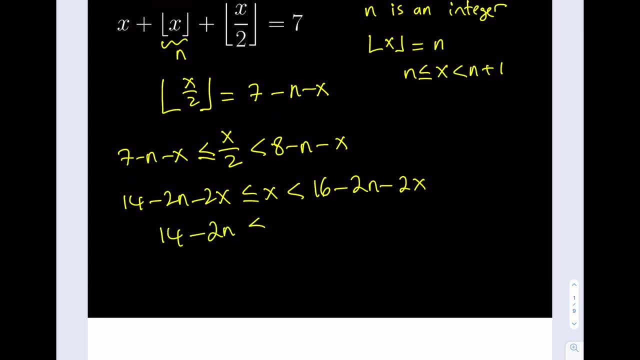 both sides. I mean 4 to everything. There are three sides, I guess. Right, Add 2x to everything, and then you should be getting something like this, which is much better than the previous. Now we've got to think about it this carefully, and I can go ahead and divide both sides by 3. 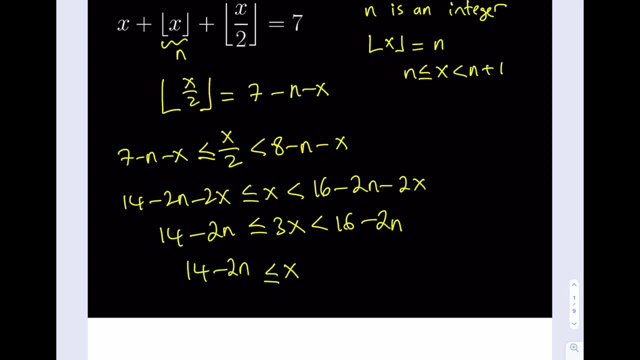 because my goal is to always get an x in the middle or somewhere Right. So now I have an interval for x, but not only I have one interval for x, I have actually two intervals for x. Why? Because at the beginning, remember, we assumed that the floor value of x is equal to n. That gave us 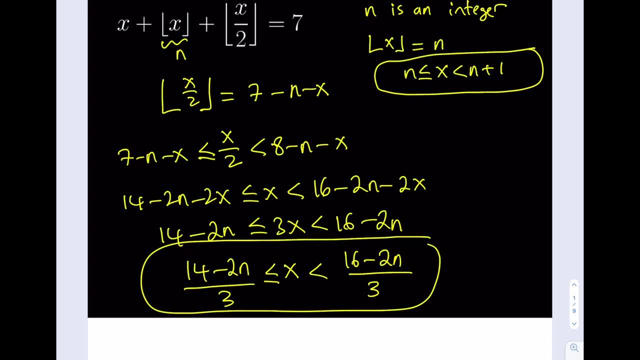 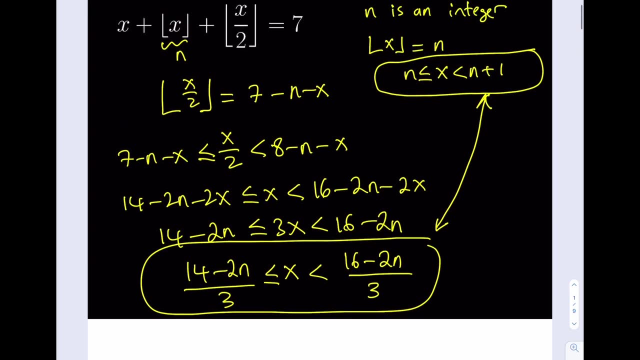 another inequality. So what we're going to do now is we're going to put these two inequalities together and then find the value of x here or find the value of n. I should say first: Right, Okay. So interestingly, I don't know why, but we're kind of getting. this is from: 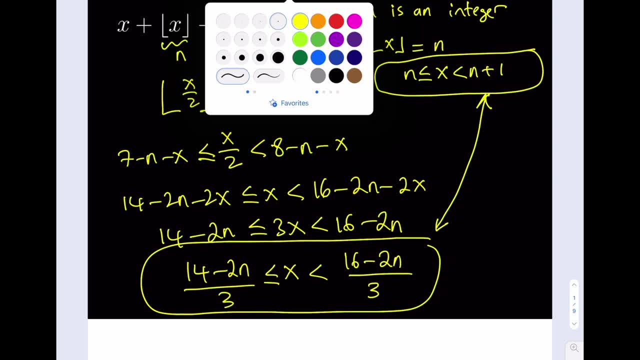 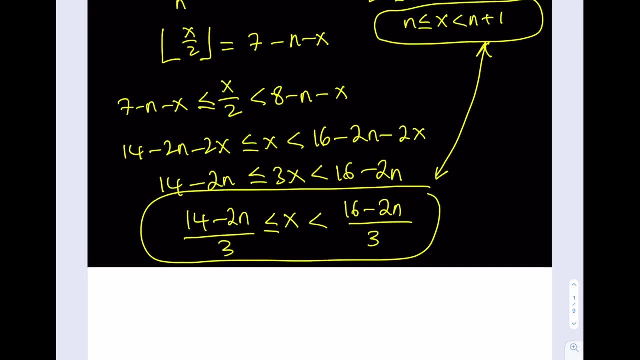 Google Docs. So we're kind of getting a different page like black and white, black and white. I guess I don't know why that's happening, but anyways, let's continue. So how do I put these together? So here's what I'm thinking Here. x is greater than or equal to something. 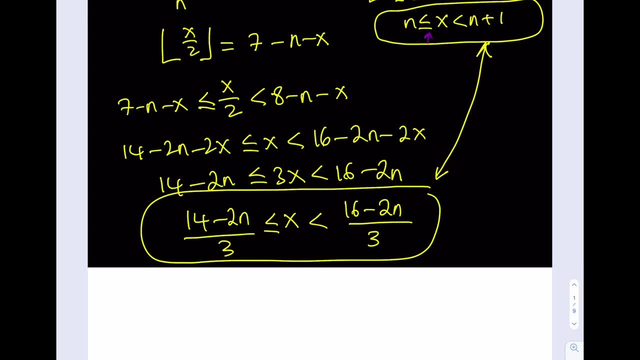 Here, x is less than something, So this value here should definitely be what. Since x is greater than that, that's a lower bound and this is an upper bound, and a lower bound should definitely be less than an upper bound. So I can safely say that n is less than 16 minus 2n over 3 and 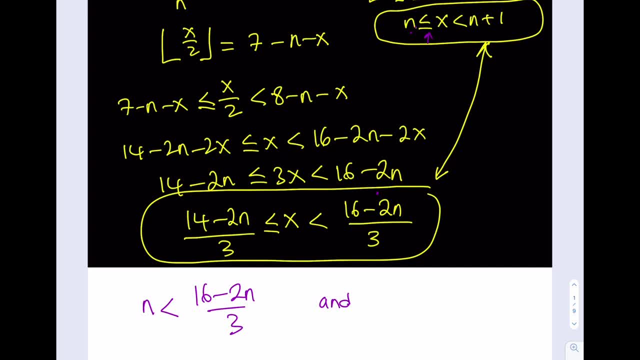 because both of these have to happen, Right? And I can say that the lower bound here, which is 14 plus 3, needs to be less than the upper bound here, which is n plus 1.. So these two inequalities have to happen at the same time, simultaneously, Right? And don't forget that n is an integer, So let's. 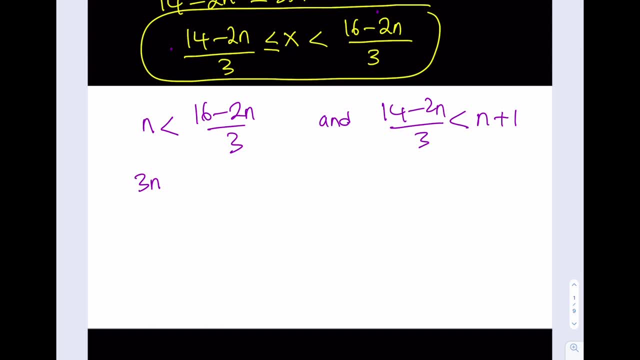 proceed? I'm going to multiply both sides by 3 and then add the 2n Right- Awesome- And then divide by 5.. Okay, Cool. So this gives me that, and on the other side, I can multiply both sides by 3 and then. 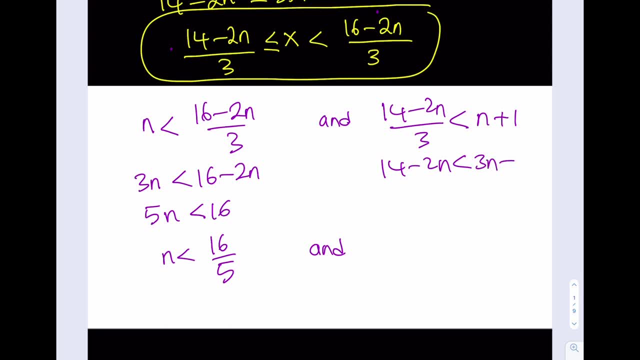 multiply by 3.. 3n plus 3.. Then what I can do is I can actually go ahead and add 2n and subtract. So this is what I'm going to be getting from here: 5n is greater than 11 and n is greater than 11. 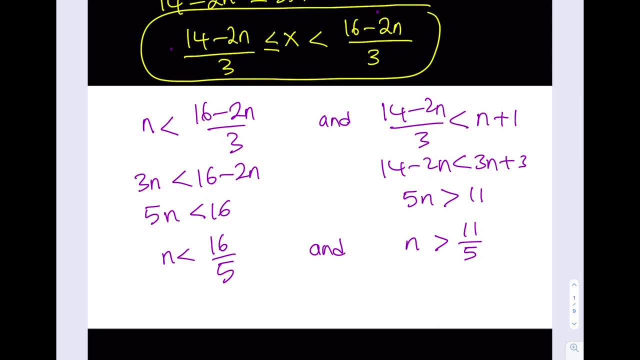 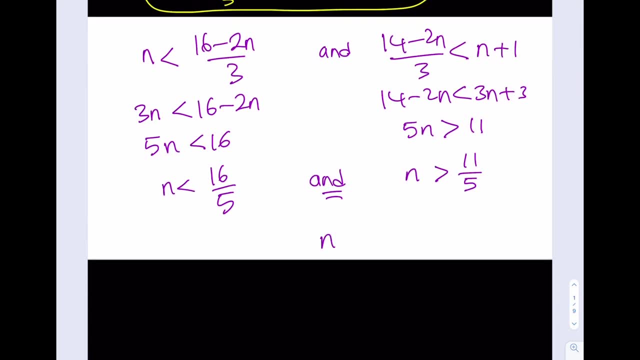 over 5.. Okay, Cool. Now, at this point, you're thinking: I have an n, so that's an intersection. This means n needs to be between 11 over 5 and 16 over 5.. Correct, Okay, Awesome. Now what am I going to do? Well, I'm going to put these together. 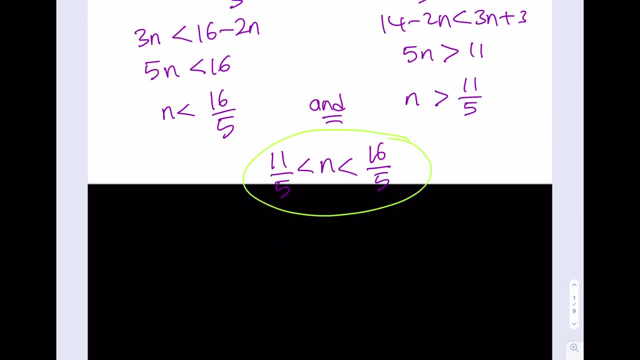 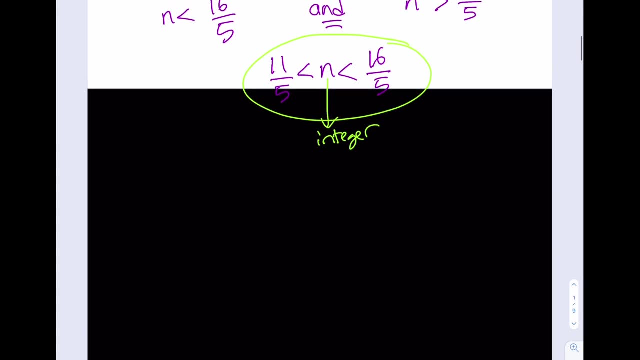 while I already did Right. So this is my conclusion. But don't forget: n is an integer, Right. Since n is an integer, what are we supposed to have? We're supposed to have a single value here. Okay, 11 point. 11 fifths is 2.2.. 16 fifths is 3.2.. So between those two values, 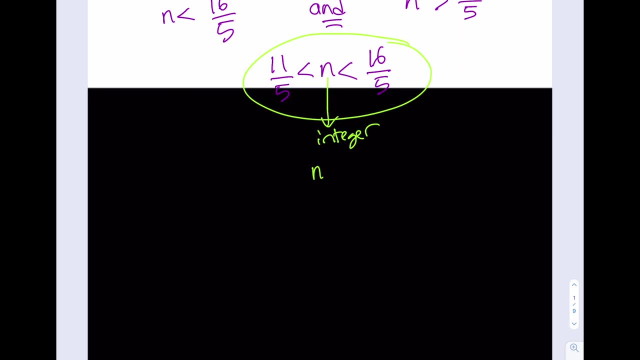 we only have one integer. So n is greater than 11 over 5.. So n is greater than 11 over 5.. So n needs to equal 3.. Awesome, But that's not the end of the story. Why? Because we need to. 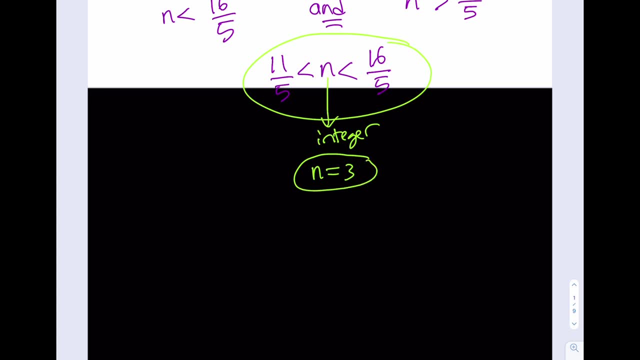 find x, But at least we were able to find a particular value for n. So this is how the floor value equations usually go: We find the value of n and then from there we're going to try to find the value of x, which could end up being an inequality Right, Okay? So what we're? 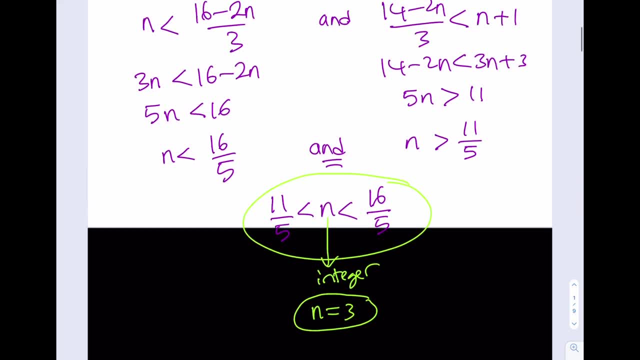 going to do next is basically the following: We're going to go ahead: take this n value, which is n, And we're going to take this n value, which is n, And we're going to take this n value, which is n equals 3.. And we're going to plug those in here and in here. Let's see what we're going to. 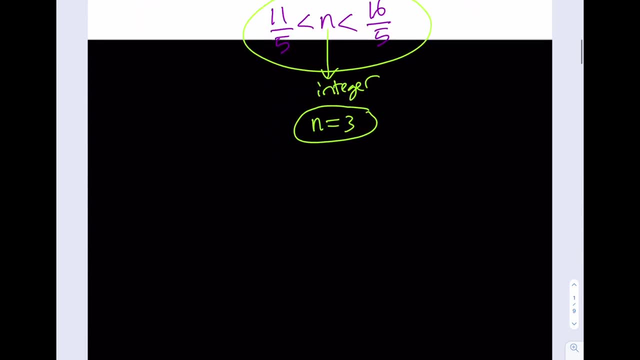 get from there. Okay, The first one is going to give me x between 3 and 4.. So this means x is between 3 and 4.. But you know, only 3 is inclusive And we have another one Right, And 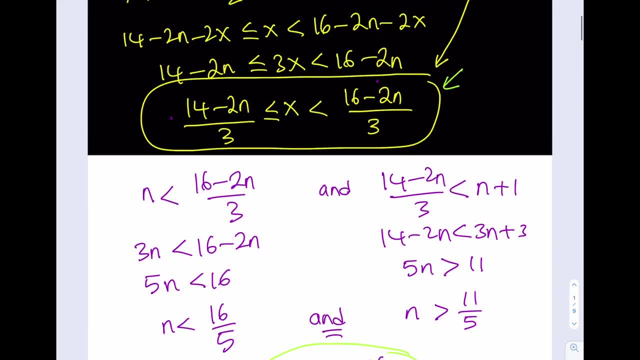 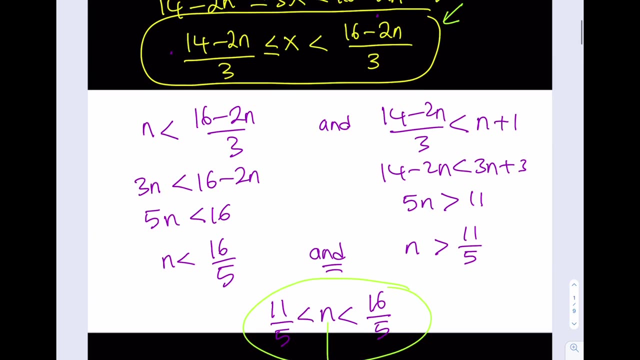 the second one gives me what? Okay. The second one gives me this: So both of them have to happen, Right? We know that both have to happen. So from here I can get x between 14 minus 2n, Right? So it's going to look like this: 14 minus 2n over 3.. So 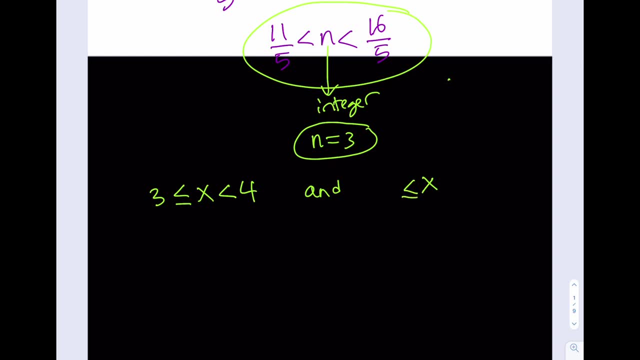 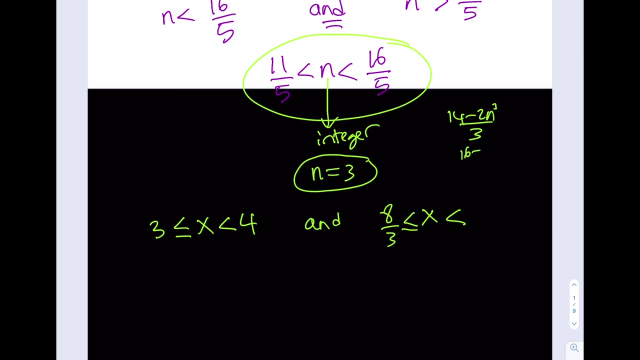 it's going to be 14 minus 2n over 3. And for that I'll use n equals 3. So that will be 14 minus 6, which is 8 thirds, And then on the other side I would have 16 minus 2n over 3. And for n equals. 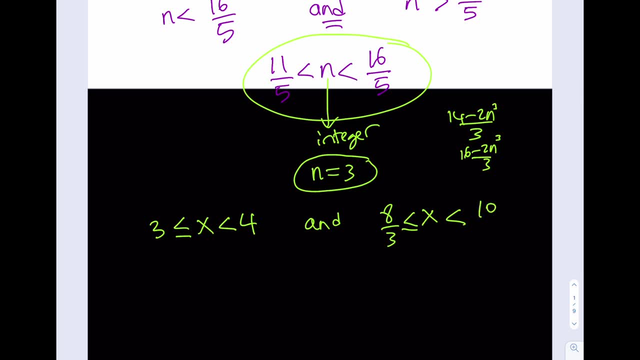 3, that would be 10 thirds. Right? So this is my conclusion: x needs to be between 3 and 4, and 8 thirds and 10 thirds. But what is that supposed to mean? Well, here's one fact. You can go ahead. 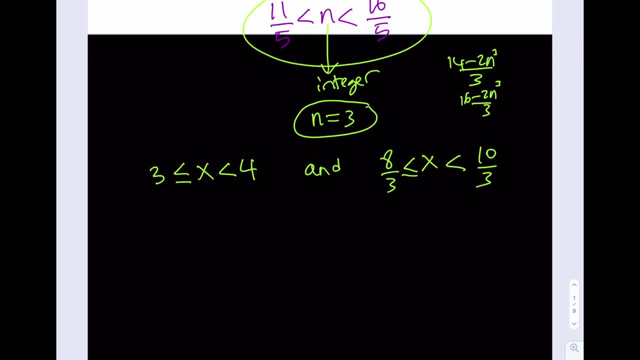 and find the intersection of these two Right, And that would mean that x is between, since this is about what? 2.6 ish Right? So this means x needs to be between 3 and 10 thirds, because 4 is greater than 10 thirds. So we need to have this. So this is my conclusion, But is that the?